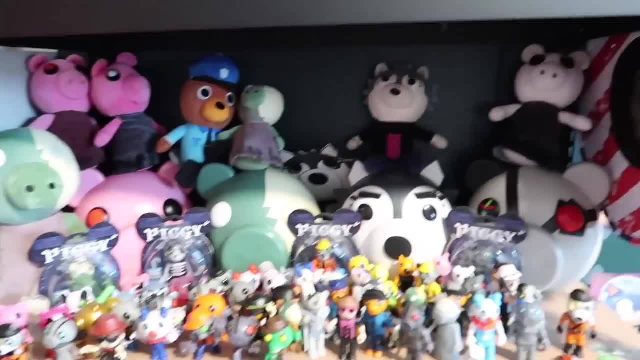 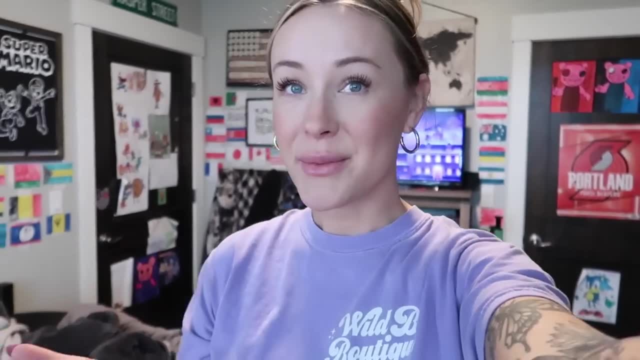 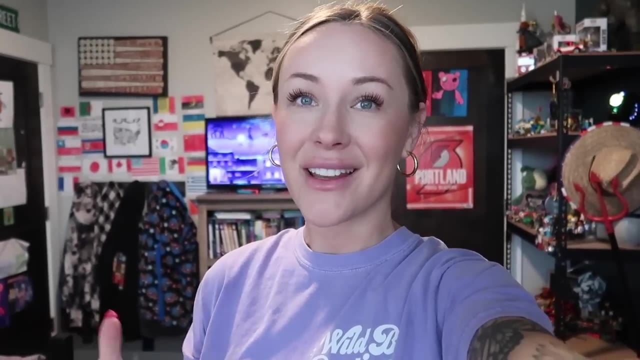 that's going to be going right there: Piggy collection, more lego stuff here, figurines and stuff. I feel like after Christmas especially, it's a really good time to go through the kids rooms and get rid of things and kind of reorganize with all their new stuff. So 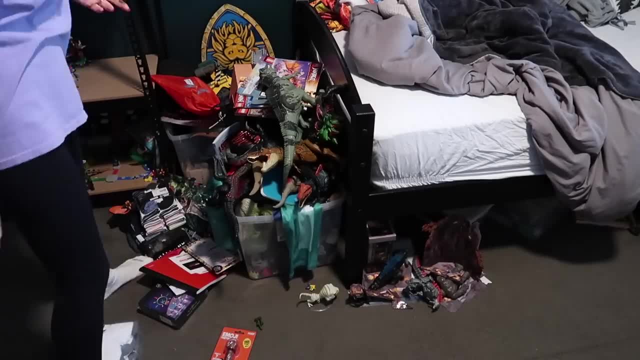 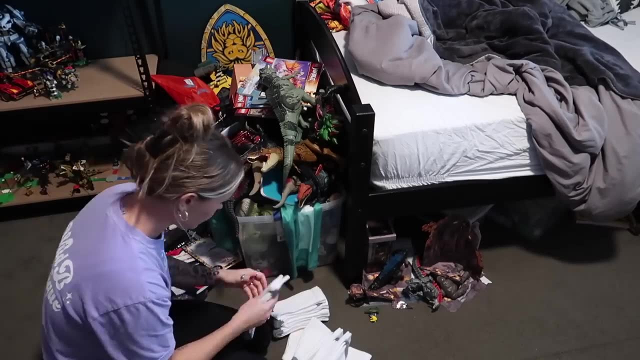 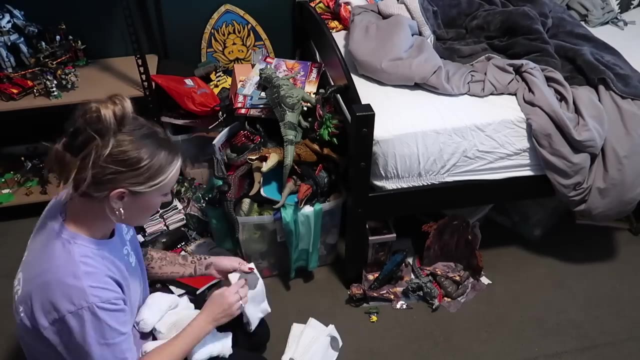 like I was telling you guys, we are working on getting all the new toys from Christmas organized along with everything else that's already in their room. So they share a room. they have lots of figurines, legos, toys, that kind of stuff. So it's just a matter of figuring out storage that works and is practical. 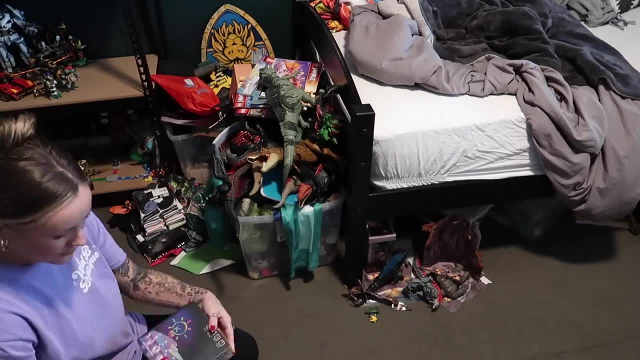 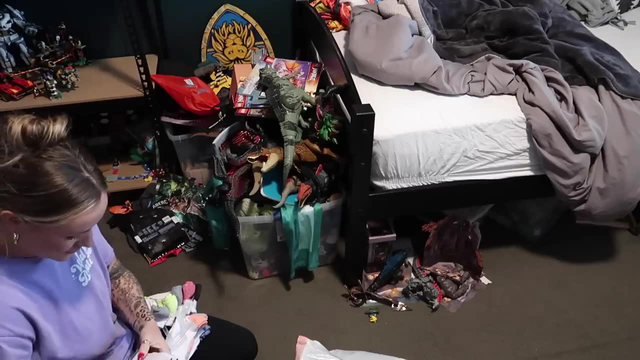 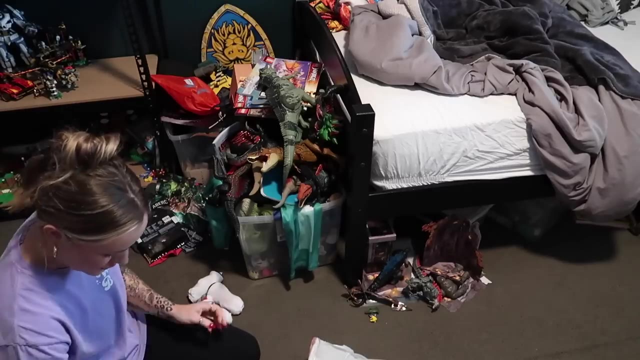 for them And they definitely have like a real life boy room and not like an aesthetic super. you know perfect room. I let them decorate how they want to decorate and let them do their thing and display what they want to display And it might seem a little cluttered. 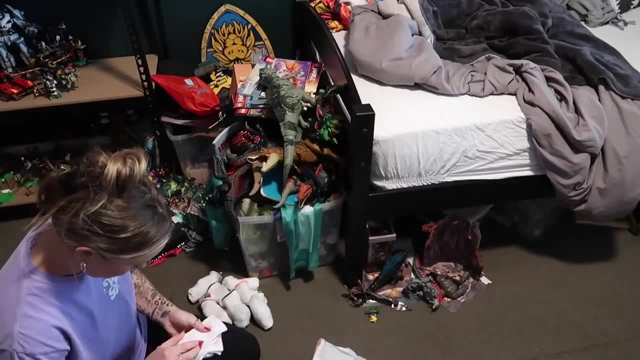 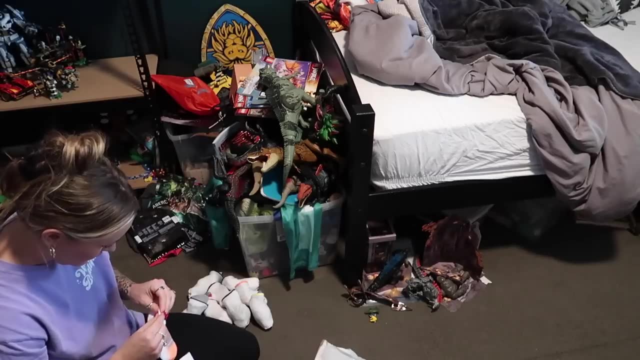 in my mind, but it's their room and they're young and I just let them do it. I let them do what they want to do with their room And they helped me along the way in this whole process, kind of behind the scenes, of figuring out rearranging and where we were going. 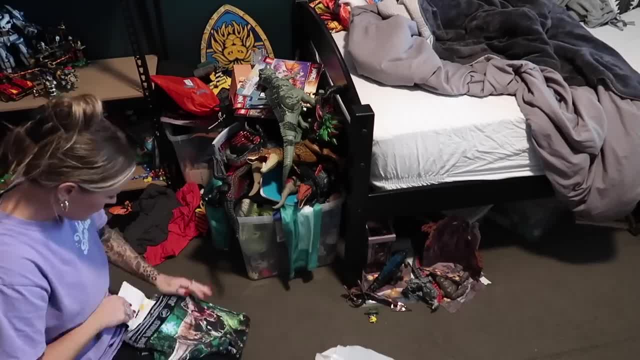 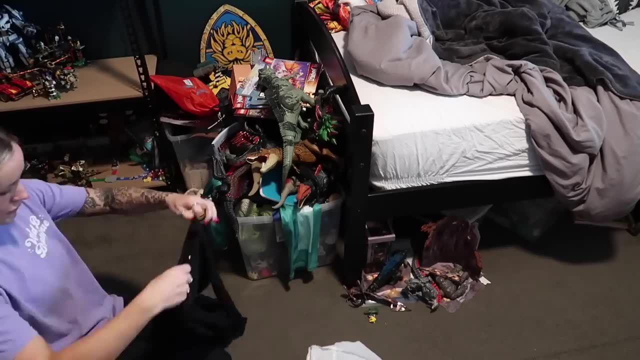 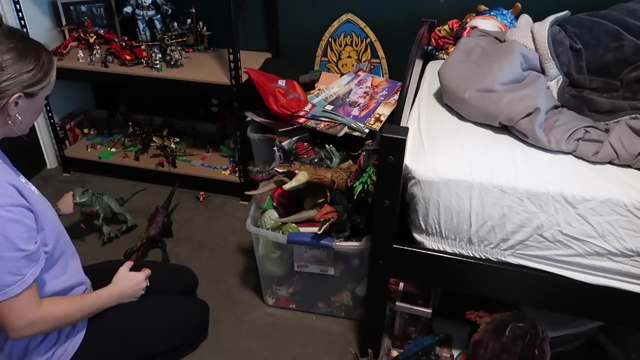 to put stuff, what we were keeping, what we were getting rid of and all of that. So, basically, I'm just starting out with these two plastic totes that we have right here at the end of one of the beds, And this started out as just a quick solution to put all of the giant dinosaur toys in. I am 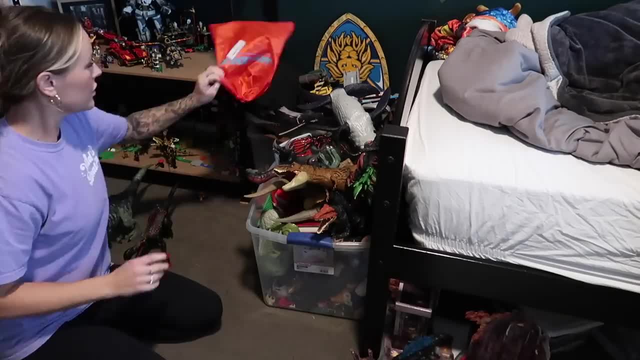 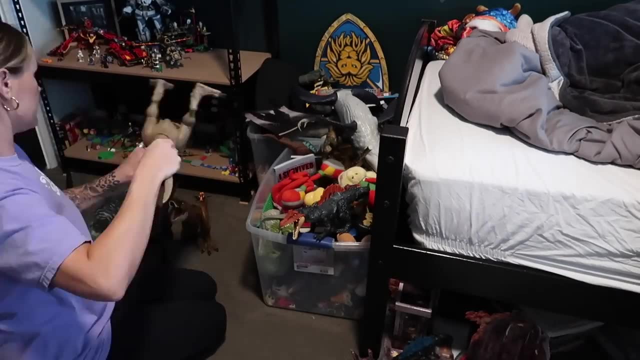 taking those out now and I'm going to set them up for Christmas. So I'm going to set them up for Christmas, I'm going to set those all over to the side. But basically what I'm doing now is just taking things out and separating them, organizing them by category Once I get everything separated. 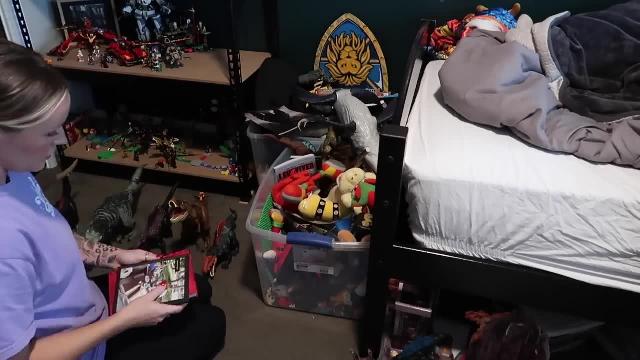 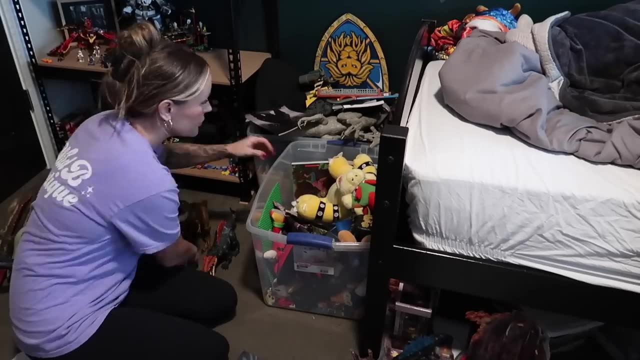 by category. I'm going to pull these clear plastic totes out of here and I'm going to replace that with a bench, a storage bench, a hope chest. actually, It's been in my family for a super long time. I believe it was my great grandma's. I should text my mom and ask her the story on it. 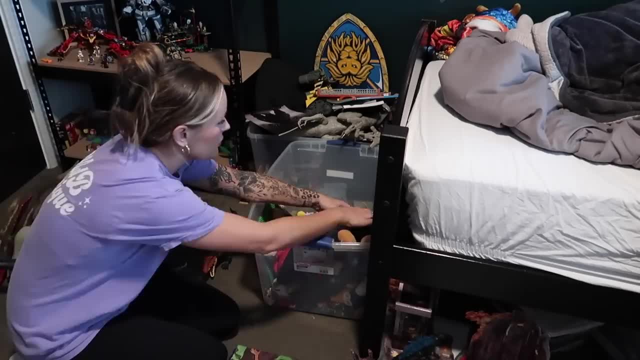 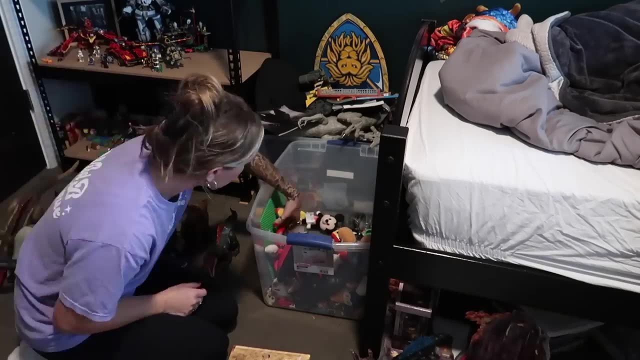 but it was passed down to me from my mom. My mom always kept blankets and stuff in it. I think I talk about that in a clip coming up, but we're going to use that as a toy box, a toy storage solution, instead of these totes. This was. 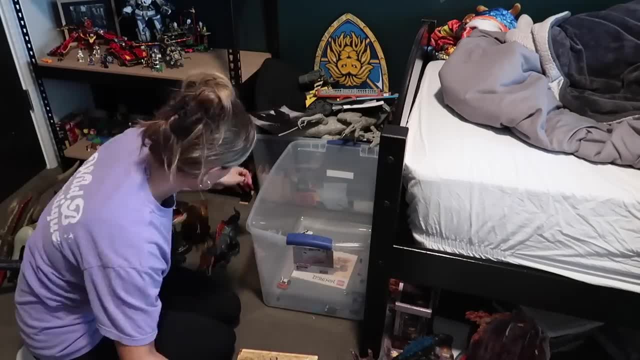 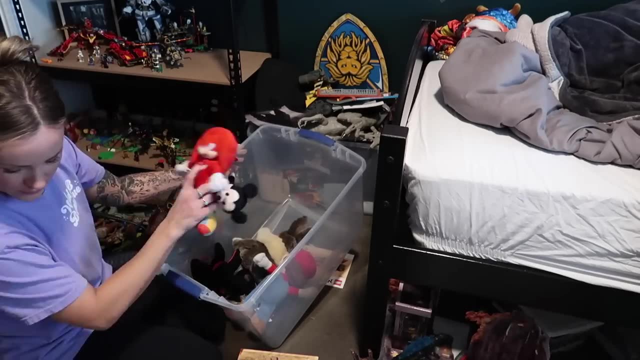 just temporary until I figured out what we wanted to do with that. And then the storage or the hope chest ended up being the perfect size to fit right here at the end of the bed and gives them a bench to sit on and gives them tons of storage for their big toys. So it ended up working out. 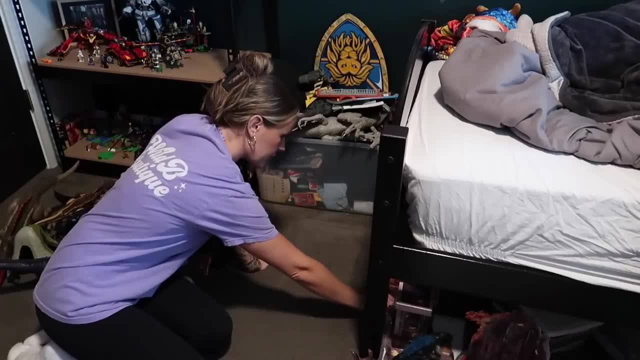 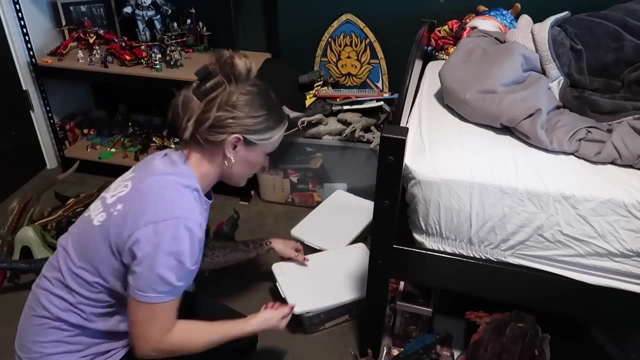 really well And I'm so happy about that. The kids are super happy about it too, So you guys will see that here shortly, but I'm just going to continue working on pulling things out from under the bed, getting things sorted out and organized. Speaker: 1 Speaker, 2 Speaker, 3 Speaker, 4 Speaker, 5 Speaker, 6 Speaker, 7 Speaker, 8 Speaker, 10 Speaker, 11 Speaker, 12 Speaker, 13 Speaker, 14 Speaker, 15 Speaker, 16 Speaker, 17 Speaker 18. 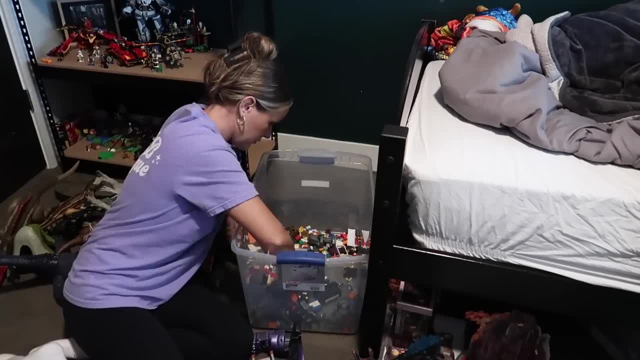 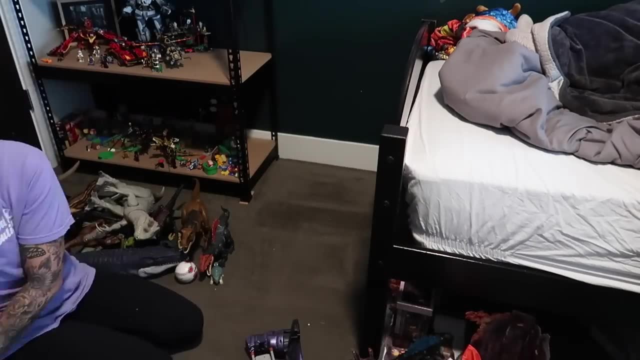 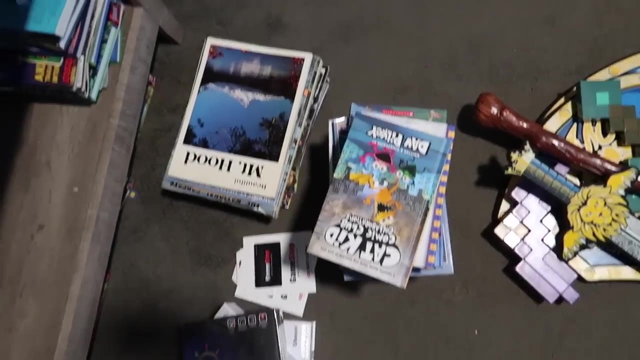 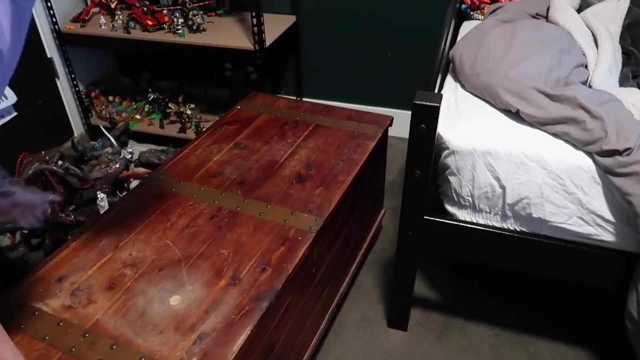 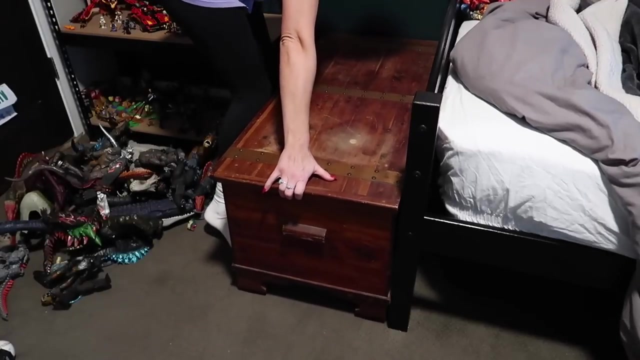 Speaker: 20 Speaker 21 Speaker 22 Speaker, 23 Speaker, 24 Speaker, 25 Speaker, 26 Speaker, 27 Speaker, 28 Speaker, 29 Speaker, 30 Speaker, 31 Speaker, 31 Speaker, 32 Speaker, 33 Speaker, 34 Speaker 35. 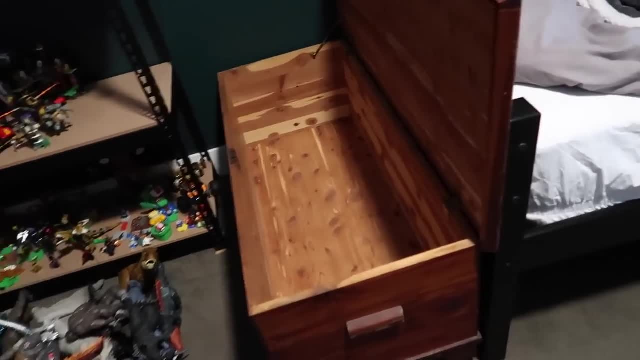 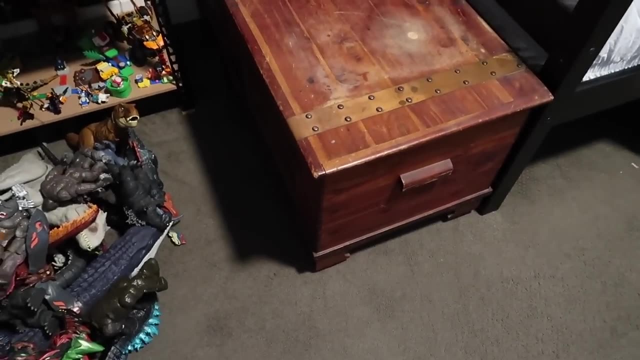 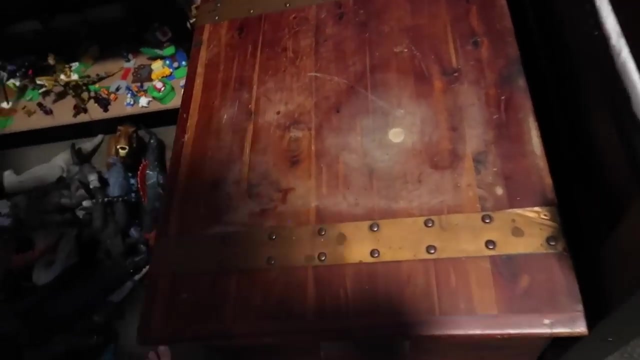 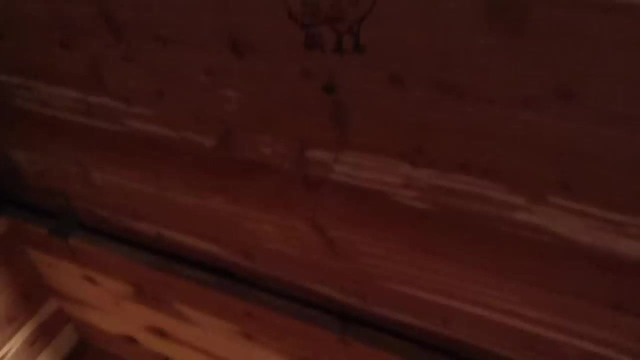 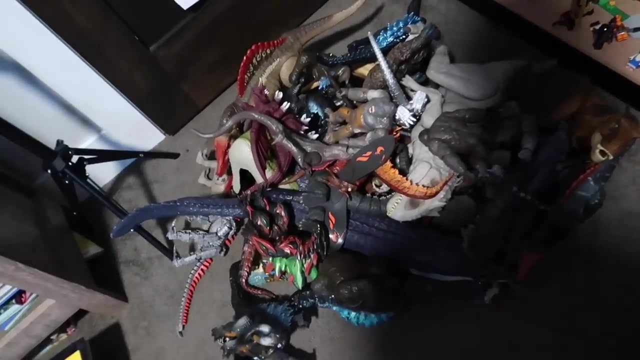 Speaker: 36 Speaker, 37 Speaker, 38 Speaker, 39 Speaker, 40 Speaker, 41 Speaker, 41 Speaker, 42 Speaker, 43 Speaker, 44 Speaker, 45 Speaker, 47 Speaker, 48 Speaker, 49 Speaker, 50 Speaker, 51 Speaker 52. Speaker: 53 Speaker, 54 Speaker, 56 Speaker, 57 Speaker, 56 Speaker, 57 Speaker, 58 Speaker, 50 Speaker, 51 Speaker, 52 Speaker. 53 Speaker, 53 Speaker, 54 Speaker, 55 Speaker, 56 Speaker, 57 Speaker 58. Speaker: 52 Speaker, 53 Speaker, 54 Speaker, 55 Speaker, 55 Speaker, 56 Speaker, 56 Speaker, 56 Speaker, 57 Speaker, 58 Speaker, 59 Speaker, 51 Speaker, 52 Speaker, 53 Speaker, 53 Speaker, 53 Speaker 54. 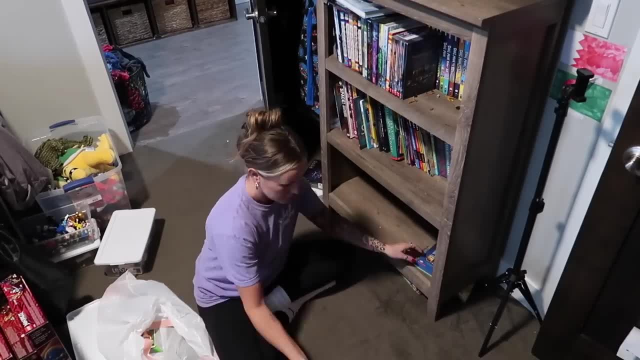 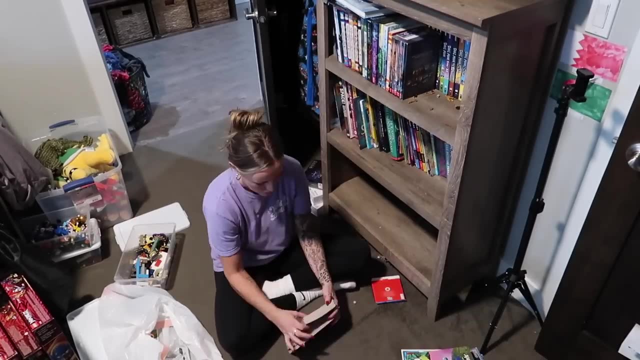 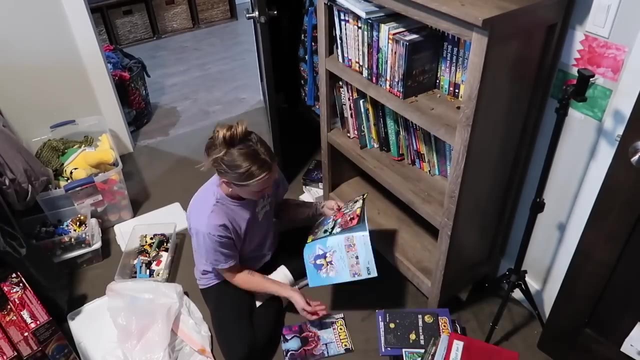 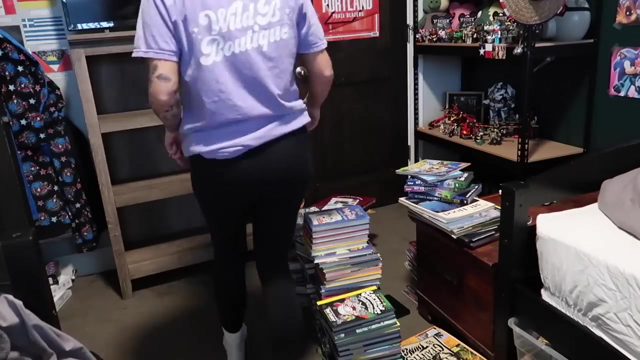 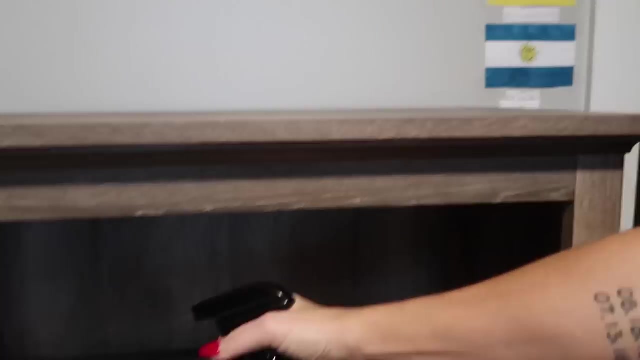 Speaker: 54 Speaker, 55 Speaker, 55 Speaker, 56 Speaker, 56 Speaker, 56 Speaker, 57 Speaker, 58 Speaker, 59 Speaker, 51 Speaker, 52 Speaker, 53 Speaker, 53 Speaker, 53 Speaker, 54 Speaker, 54 Speaker 55. 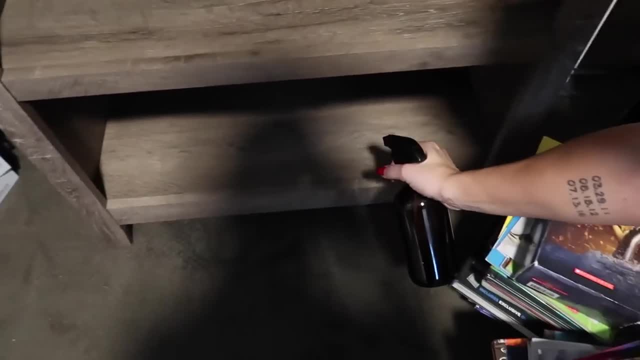 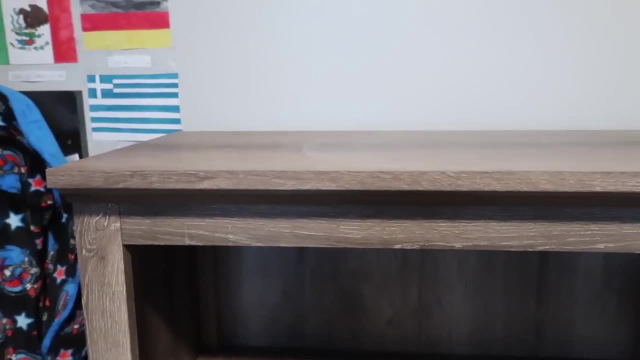 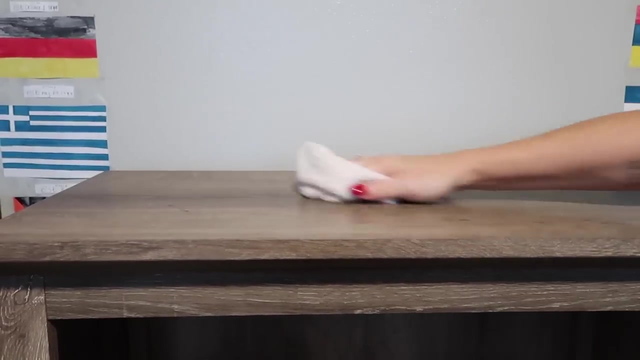 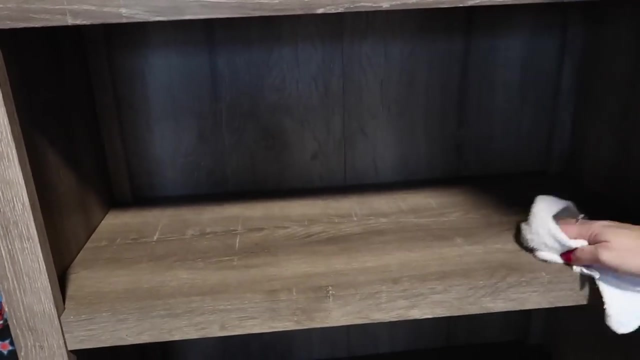 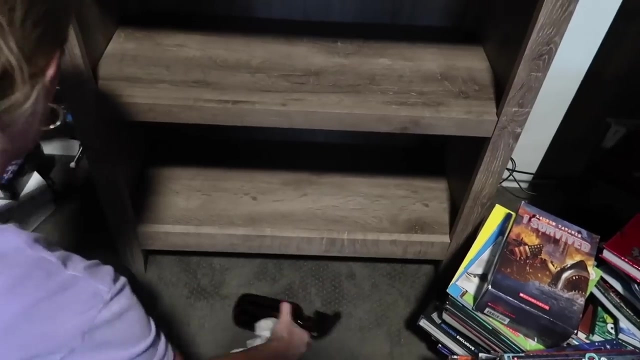 Speaker 56 Speaker 56 Speaker 56 Speaker, 57 Speaker, 58 Speaker, 58 Speaker, 59 Speaker, 52 Speaker, 53 Speaker 53 Speaker 54 Speaker 53 Speaker 54 Speaker 55 Speaker 56 Speaker, 56 Speaker 56. 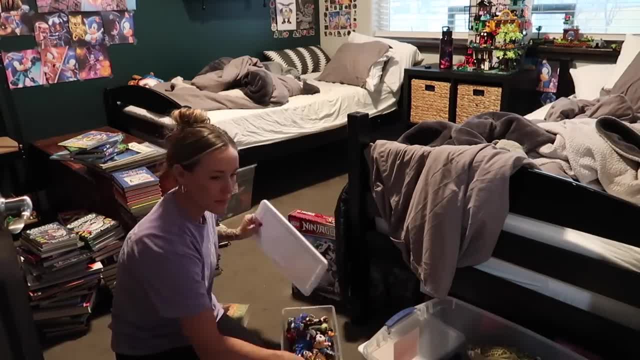 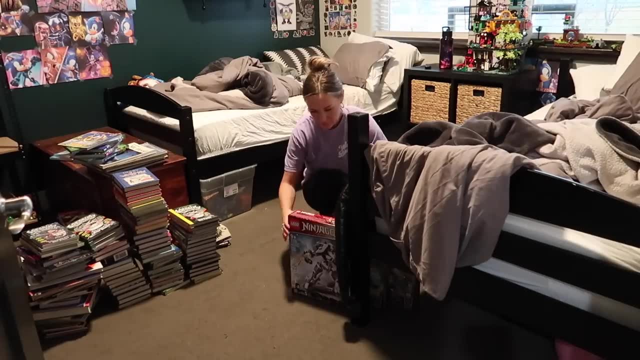 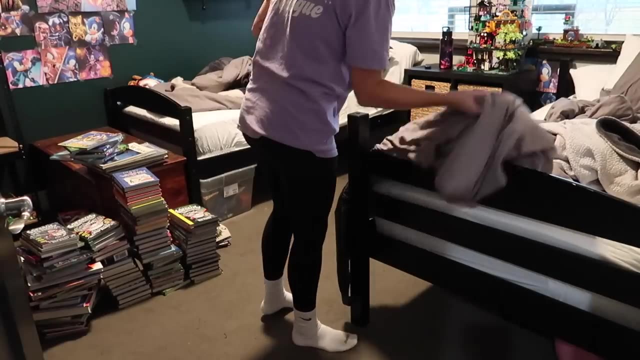 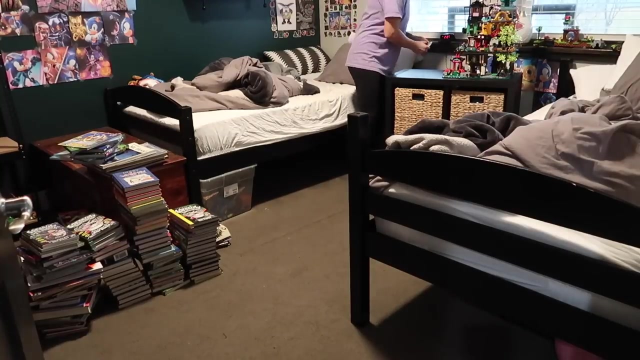 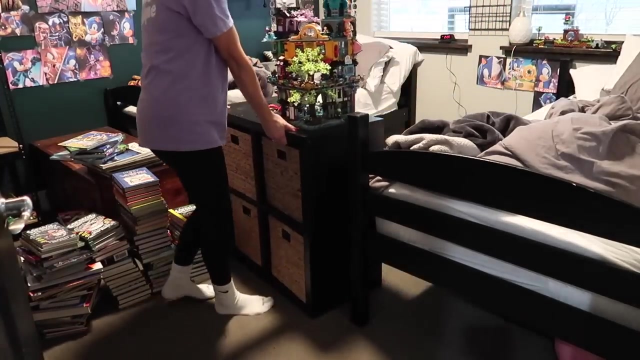 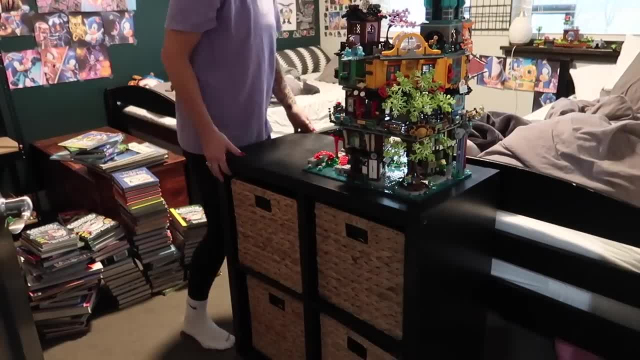 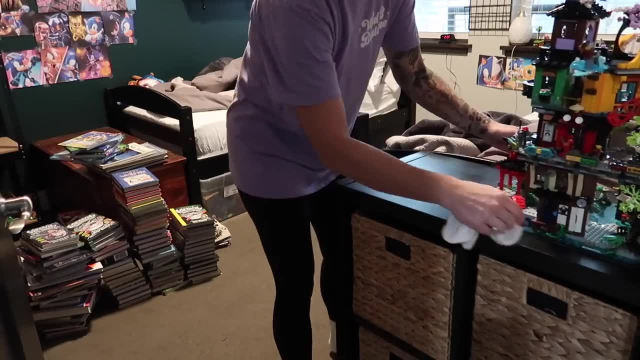 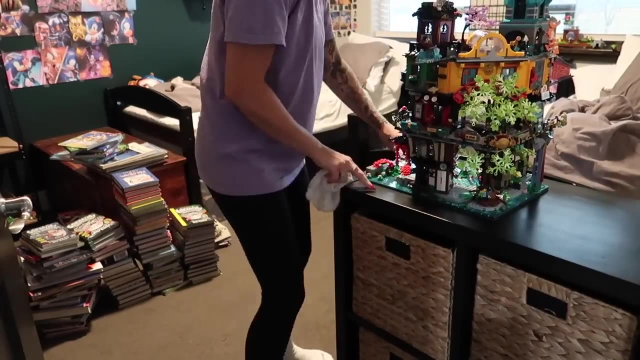 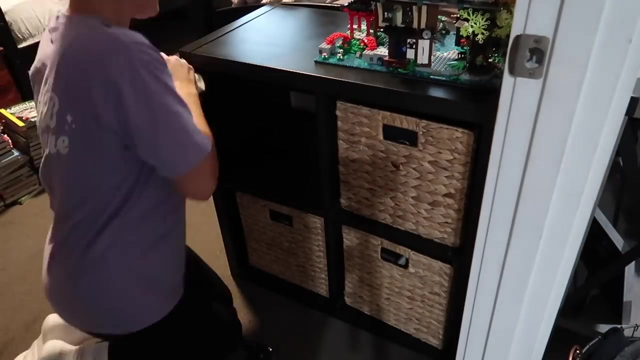 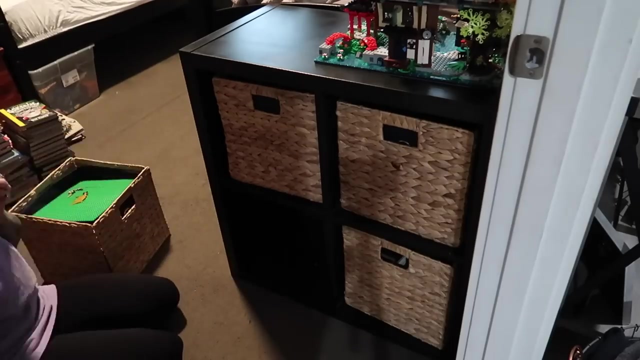 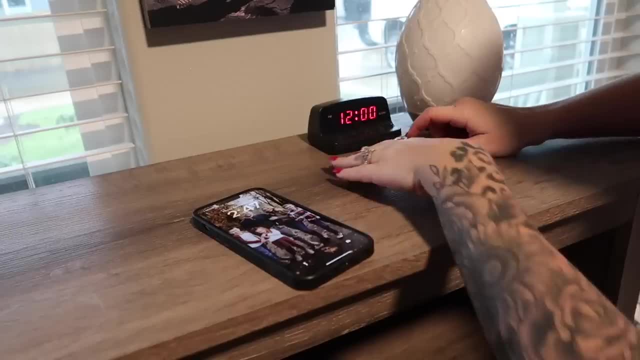 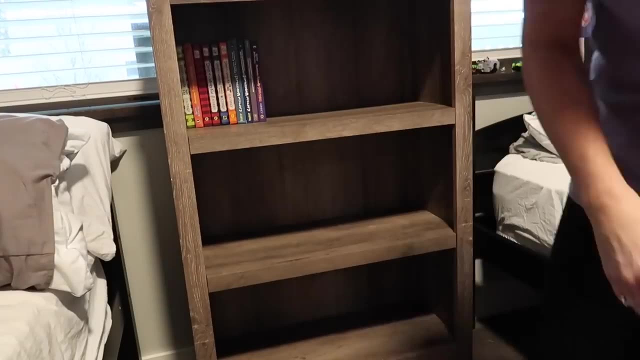 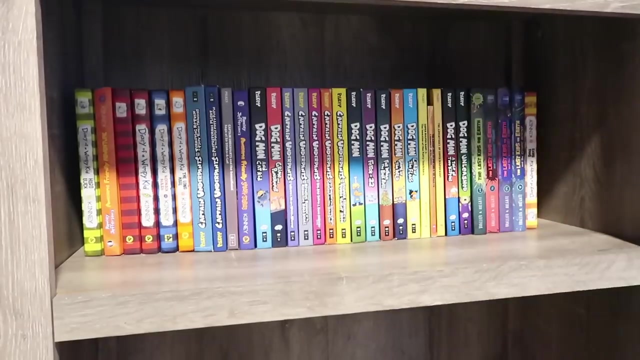 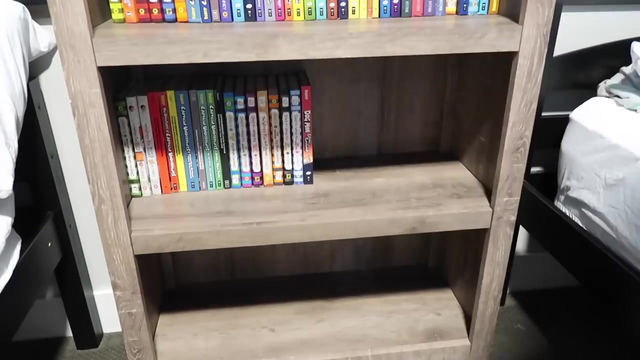 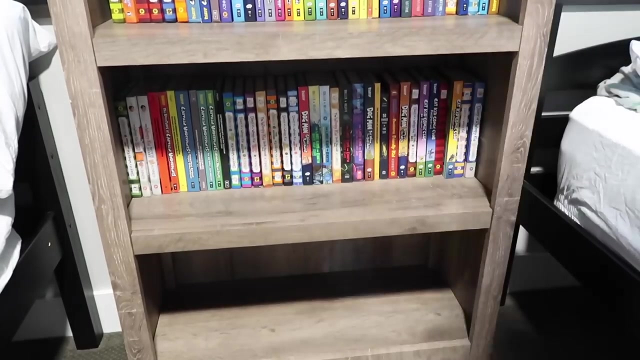 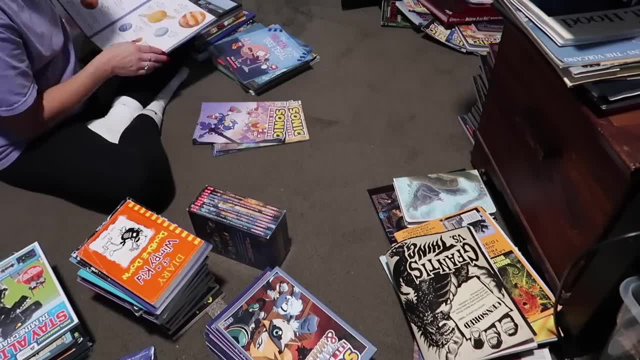 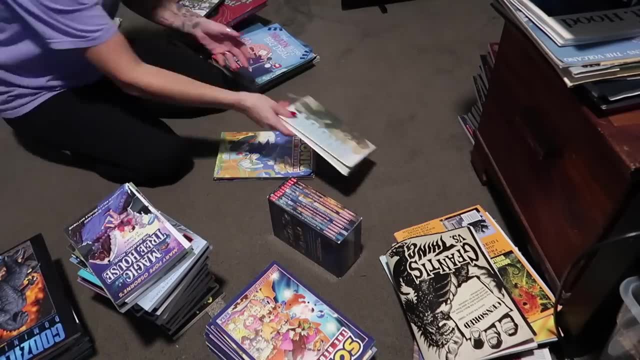 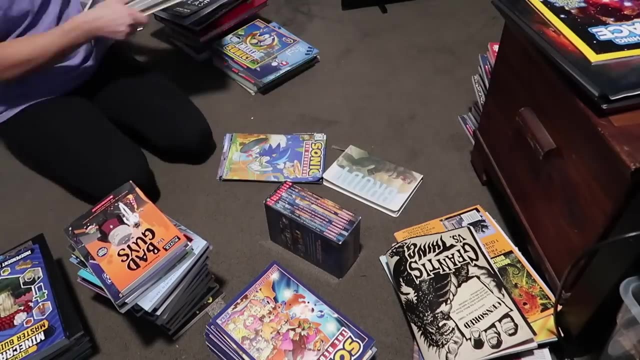 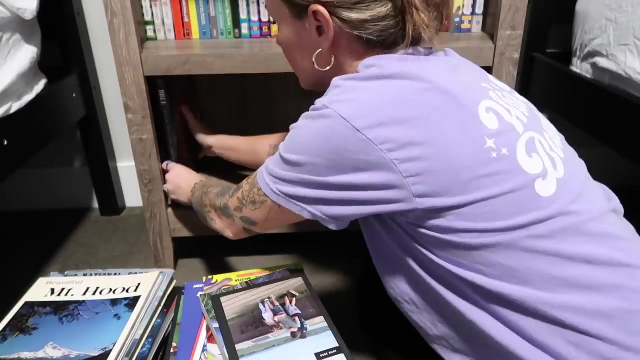 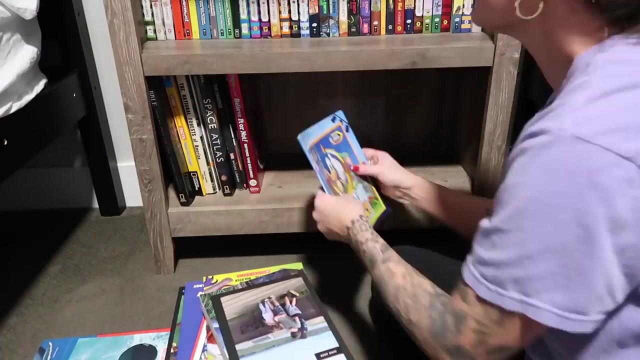 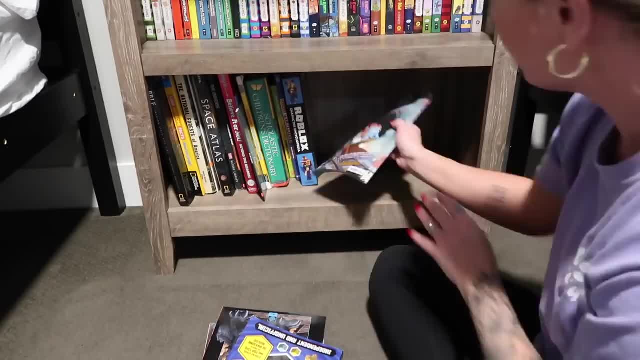 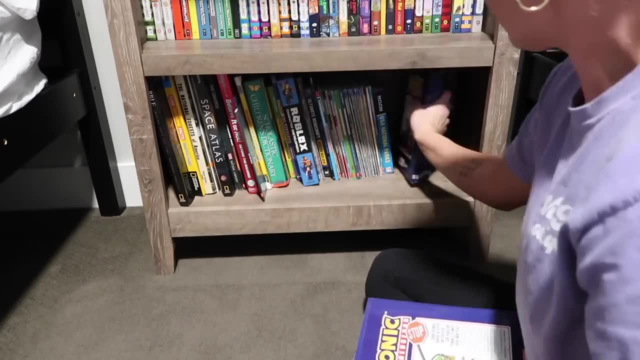 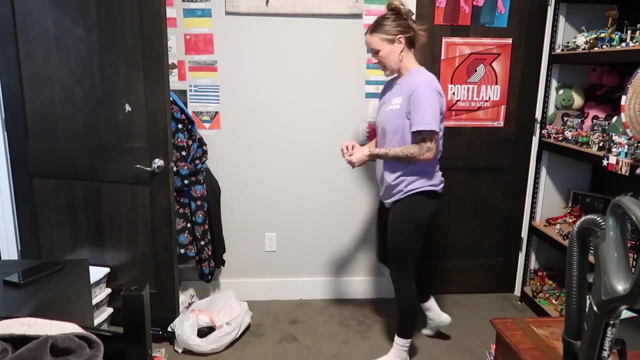 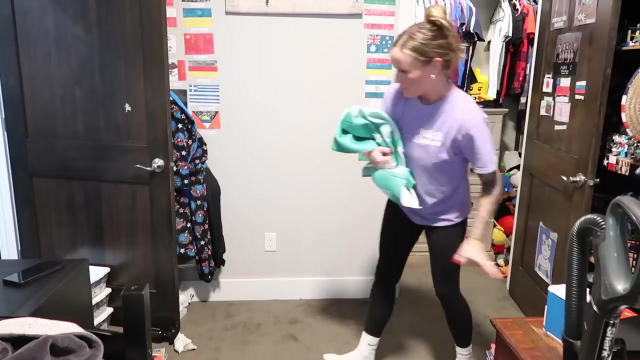 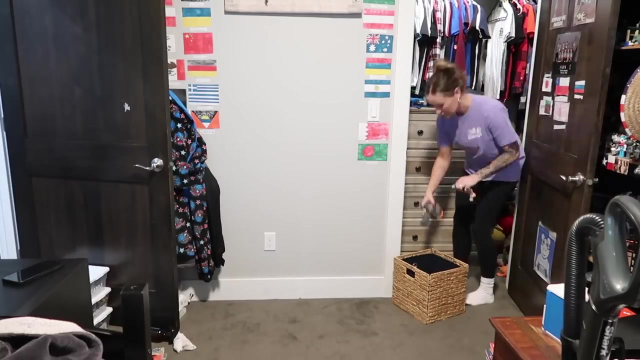 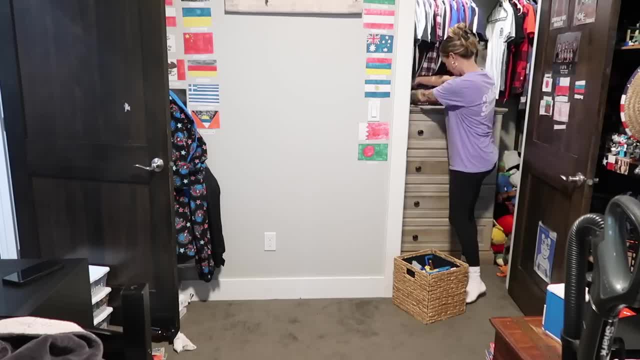 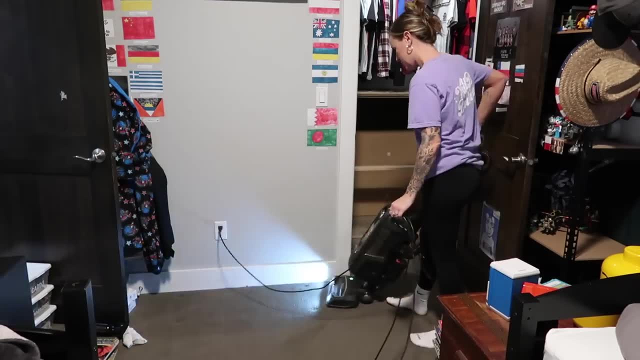 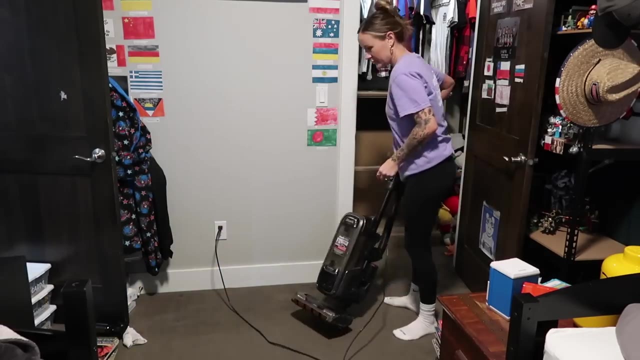 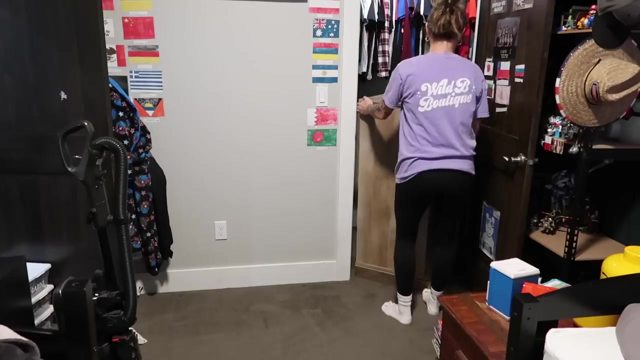 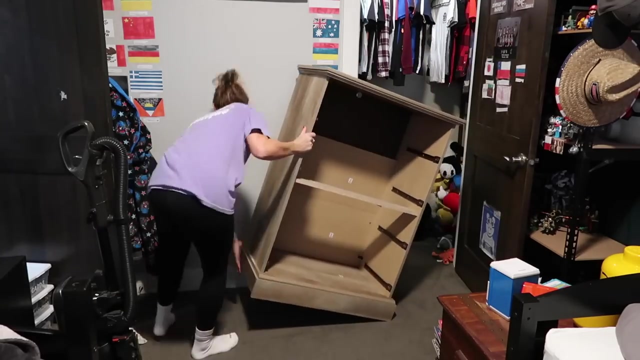 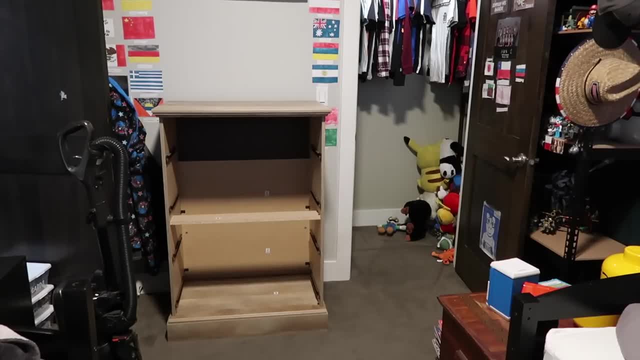 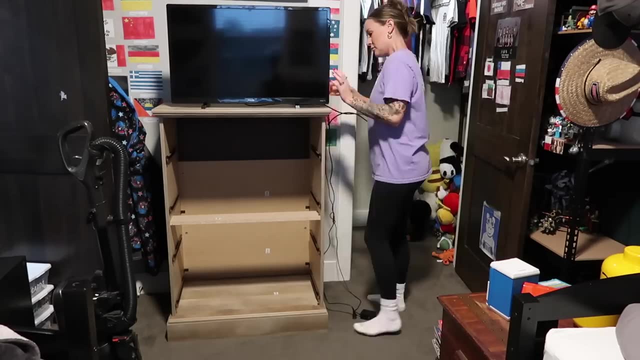 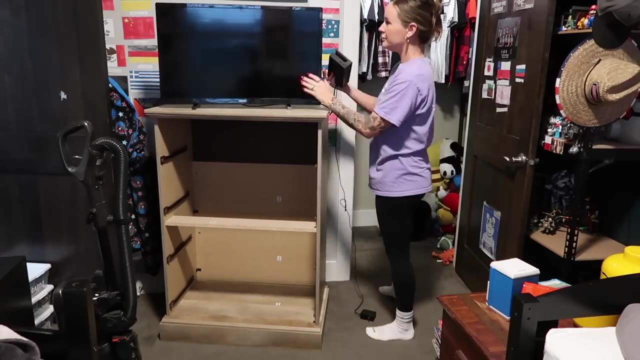 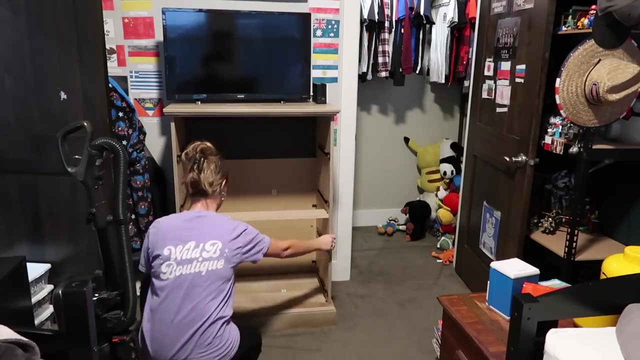 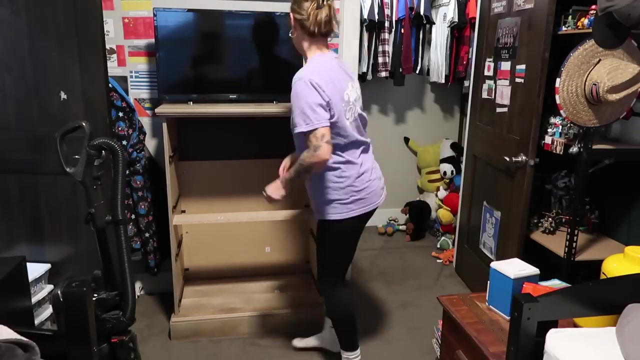 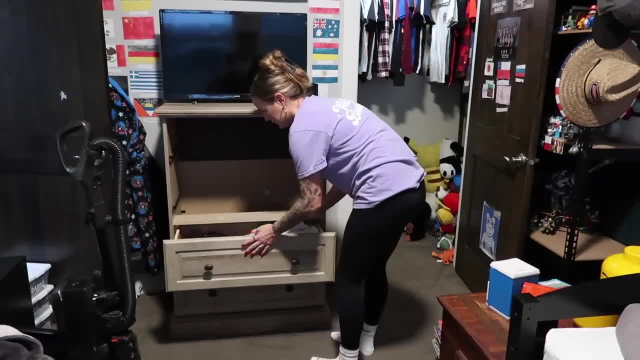 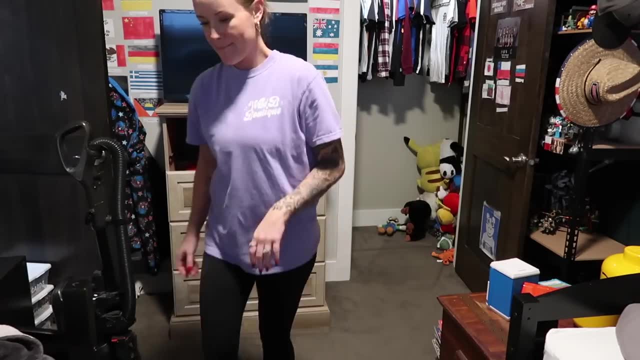 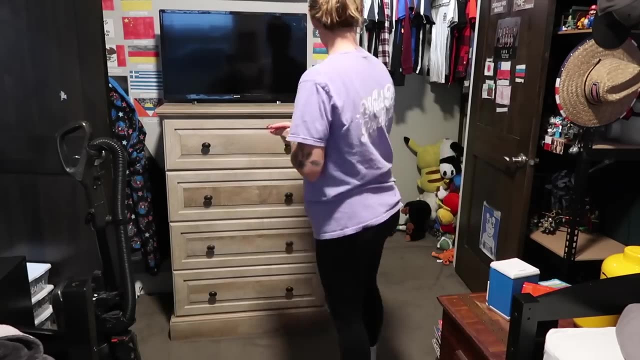 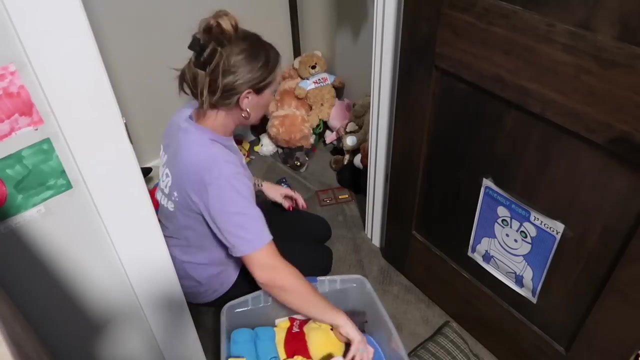 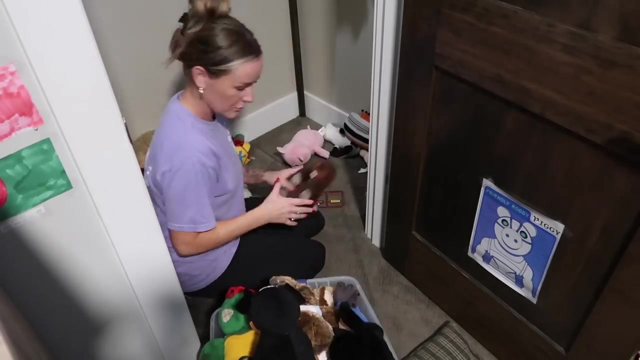 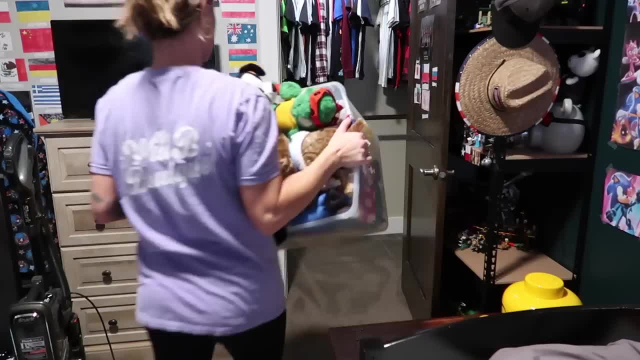 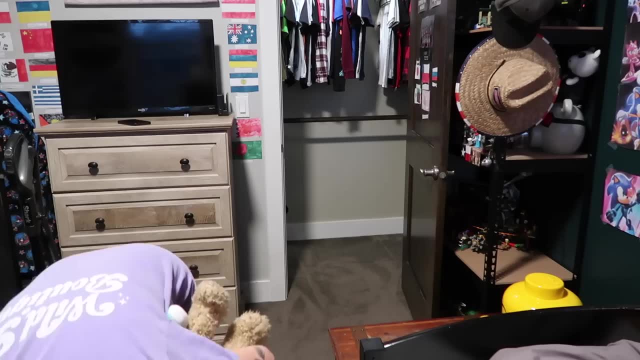 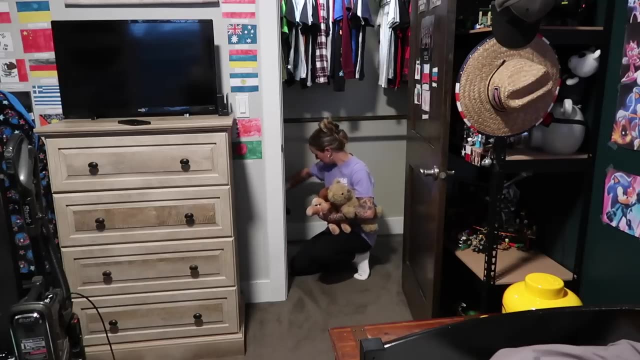 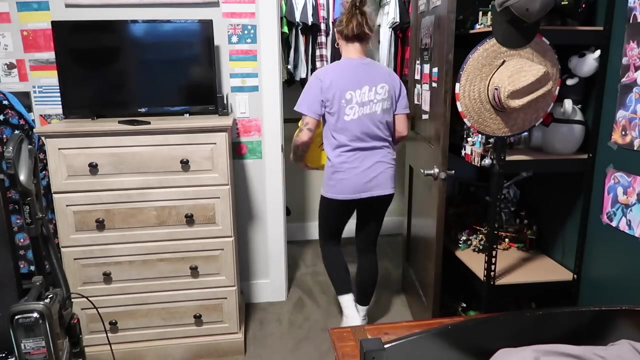 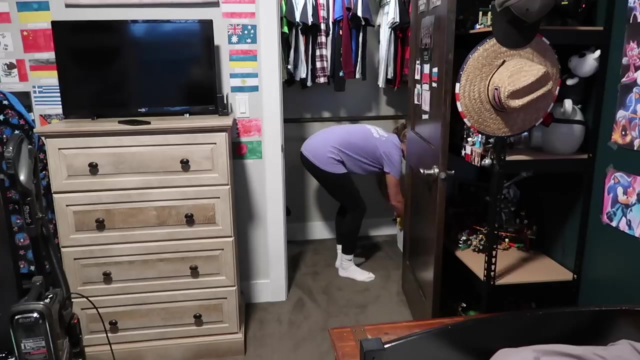 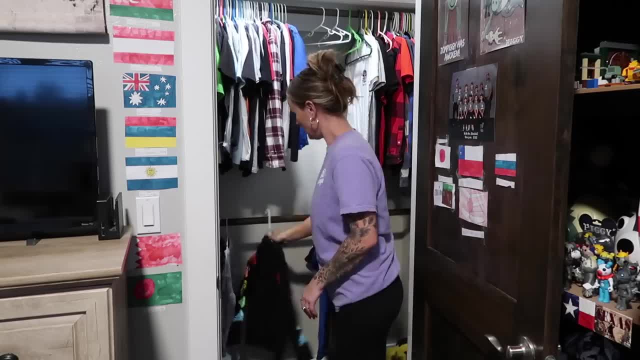 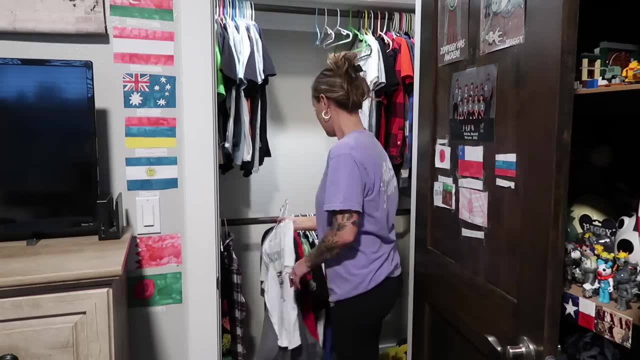 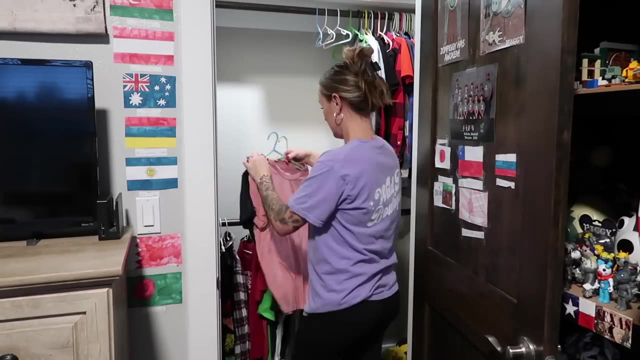 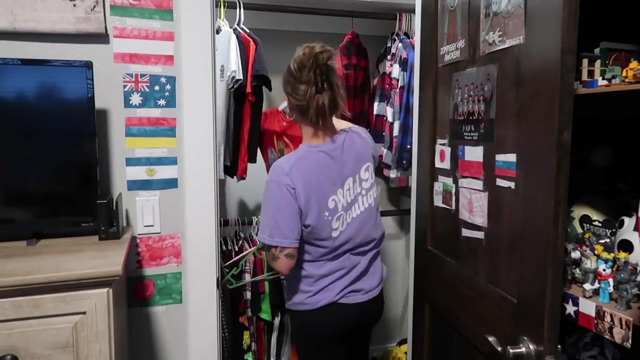 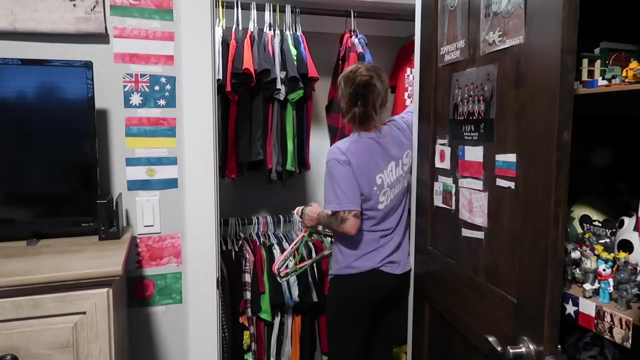 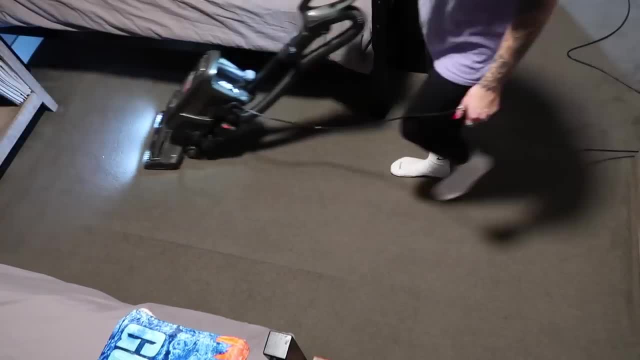 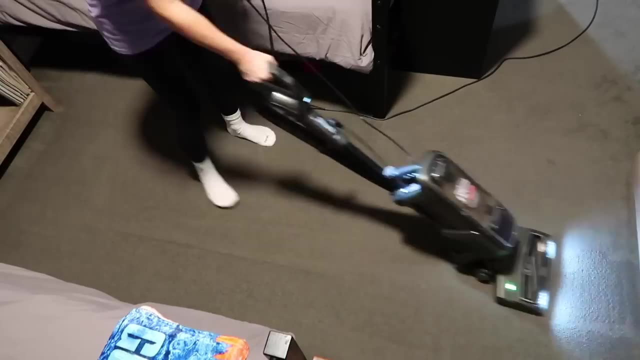 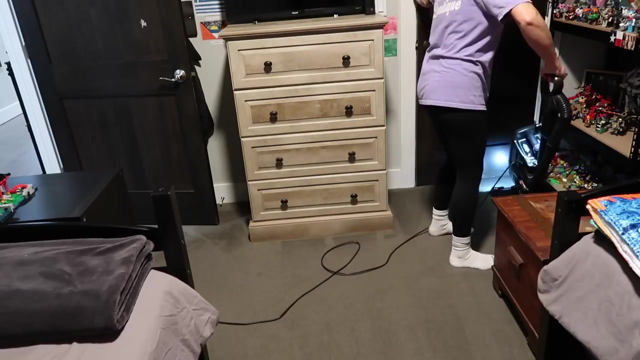 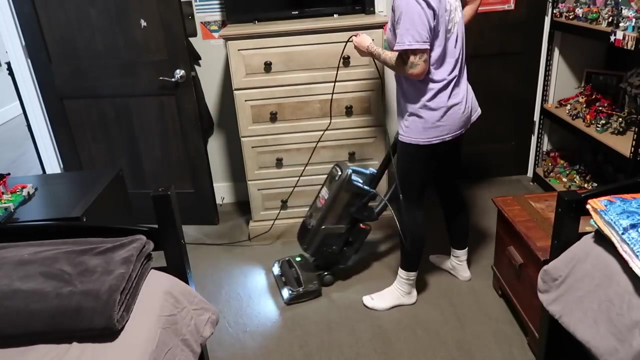 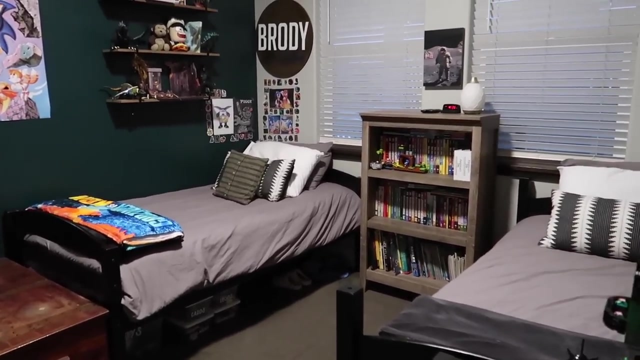 Speaker: 53 Speaker 53 Speaker, 54 Speaker, 54 Speaker, 55 Speaker, 56 Speaker, 56 Speaker, 56 Speaker, 57 Speaker, 58 Speaker, 58 Speaker, 59 Speaker, 52 Speaker, 53 Speaker, 53 Speaker, 54 Speaker 53. 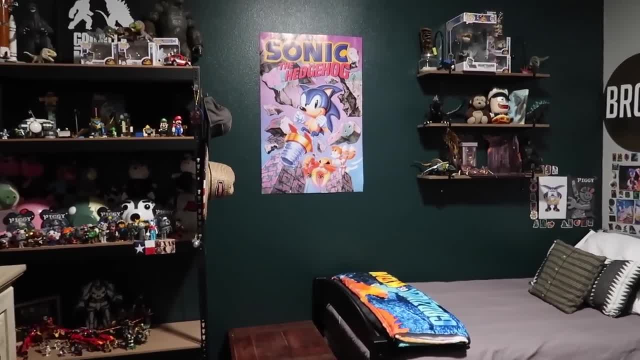 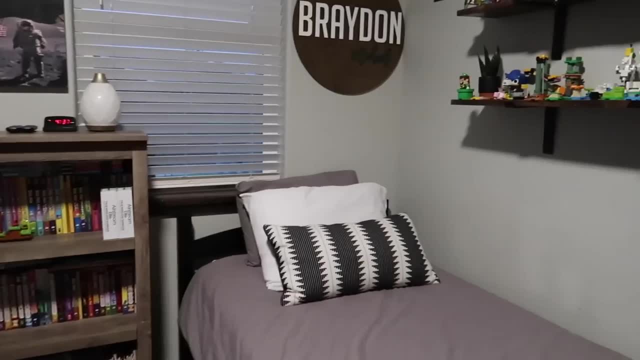 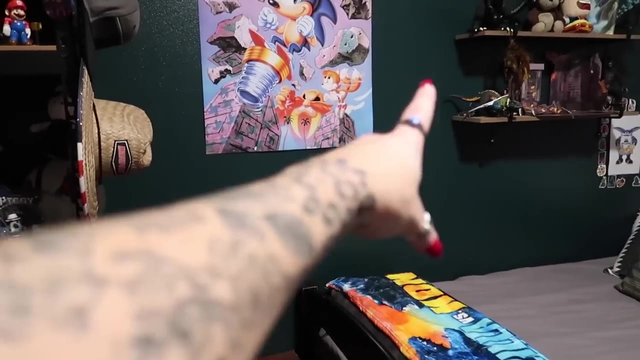 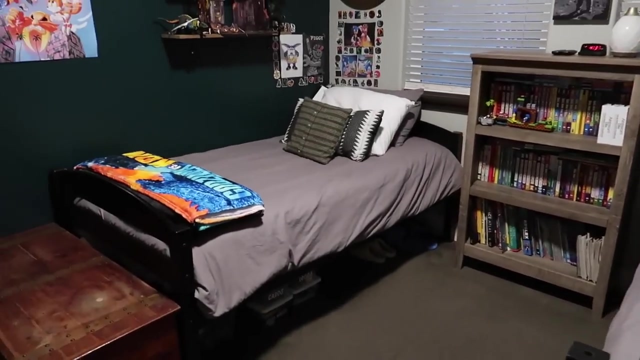 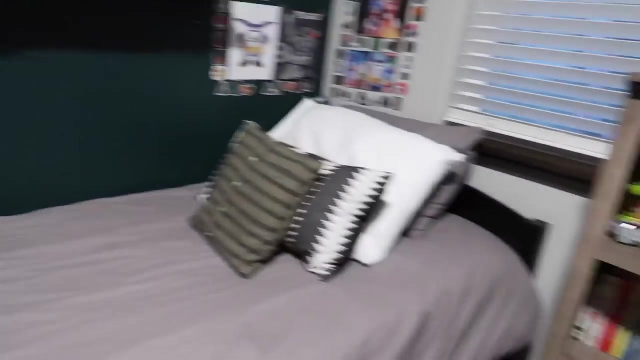 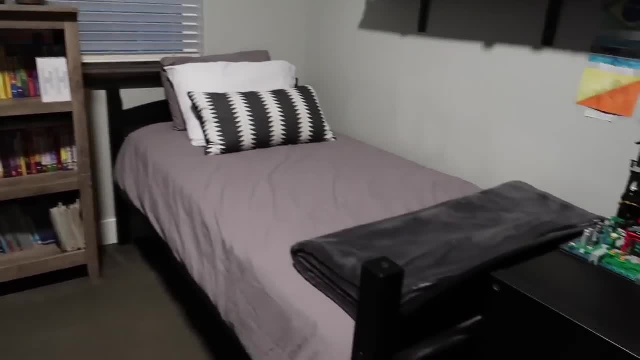 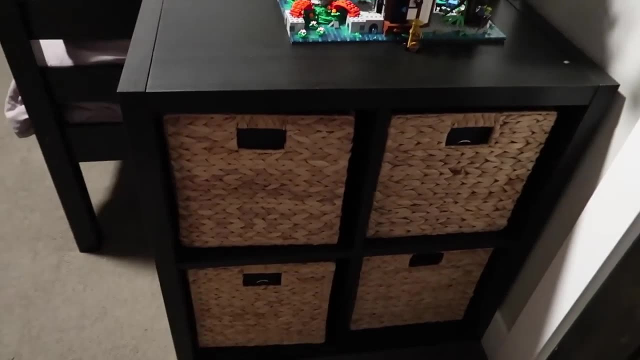 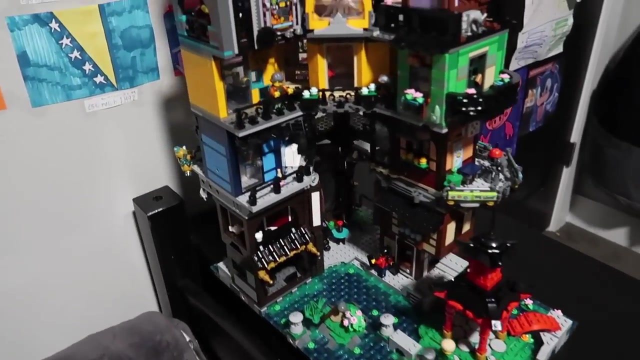 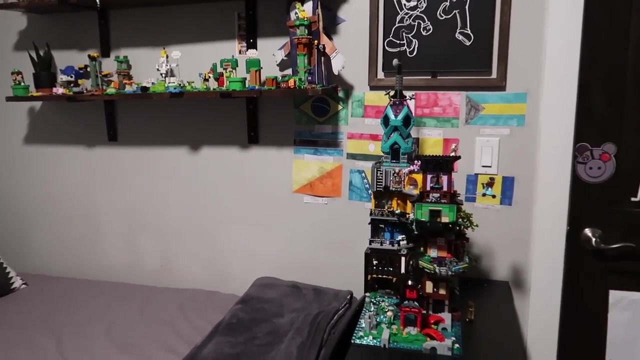 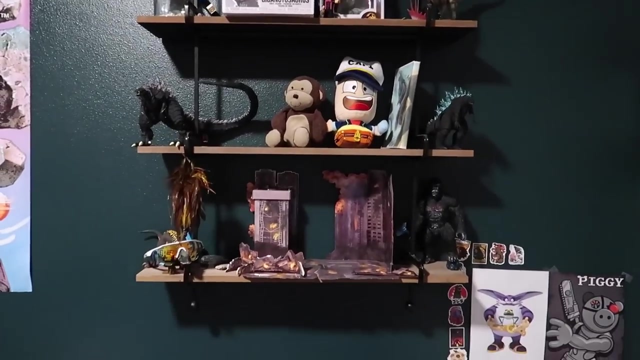 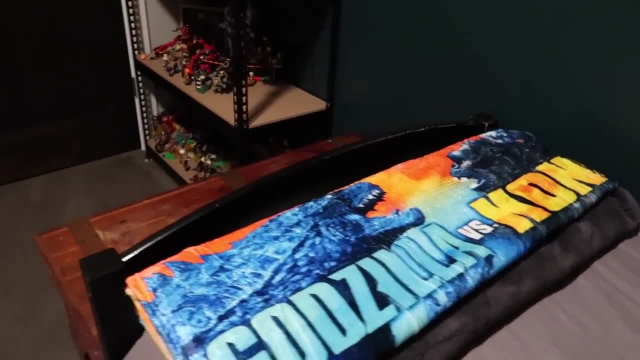 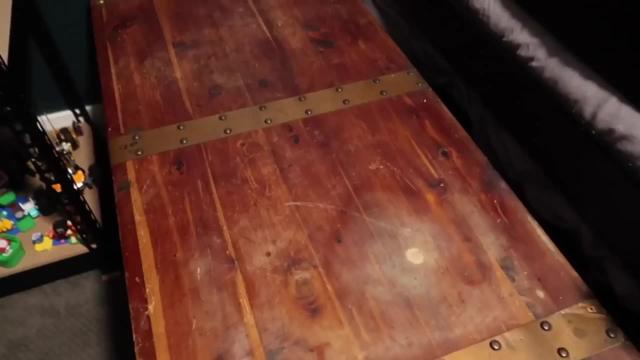 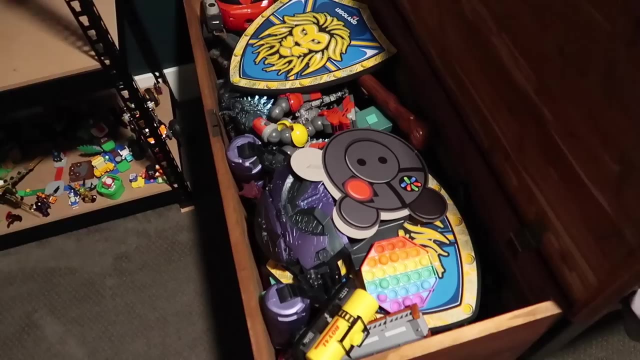 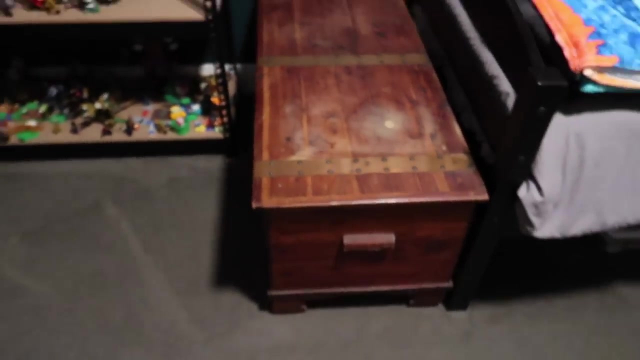 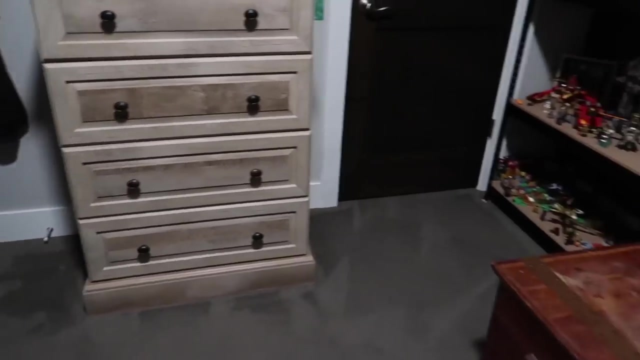 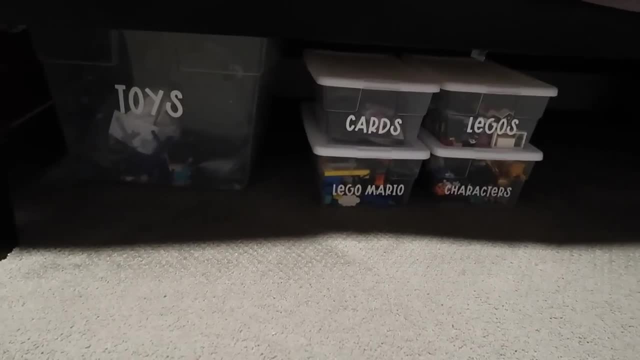 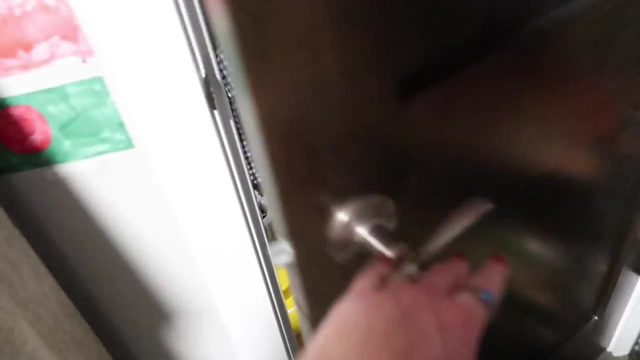 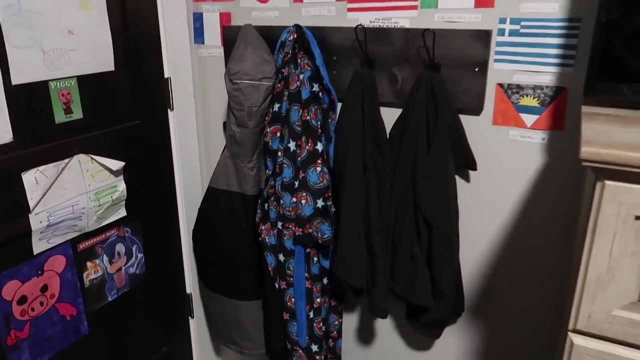 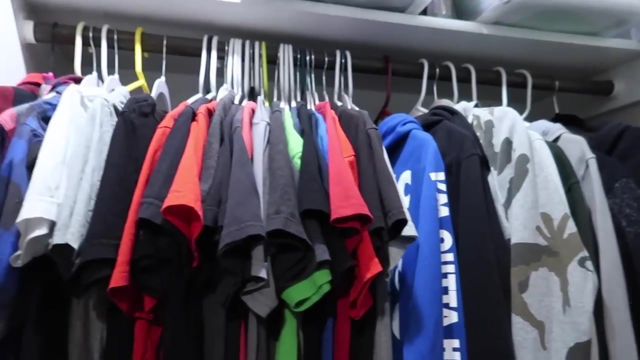 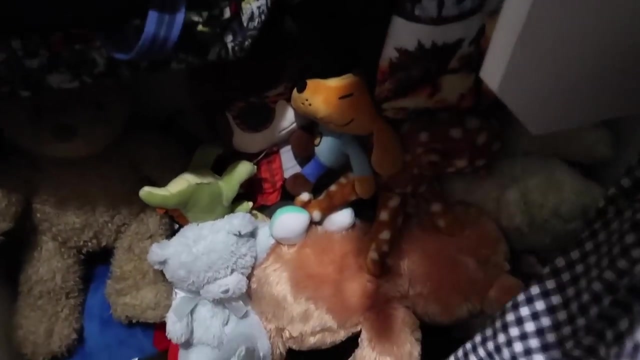 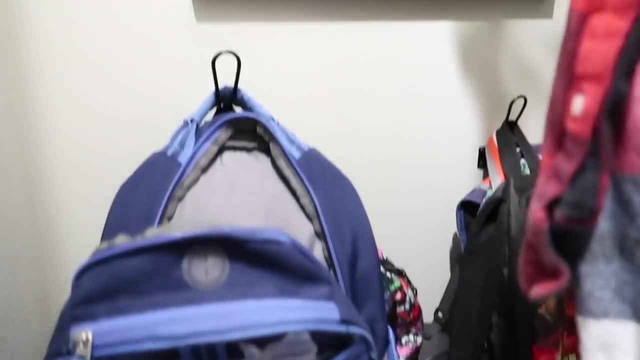 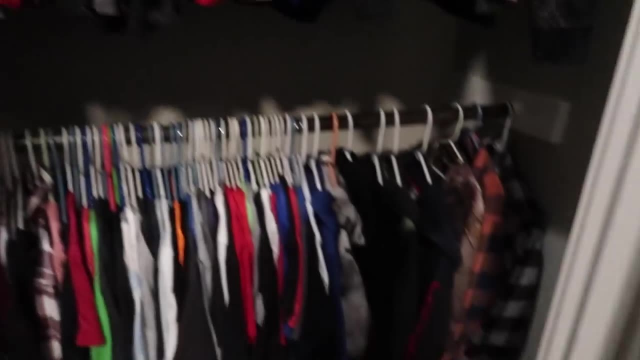 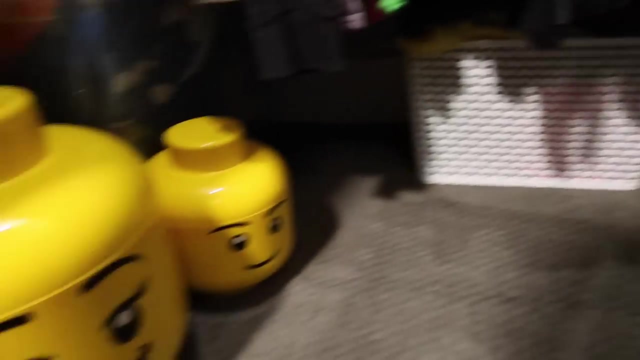 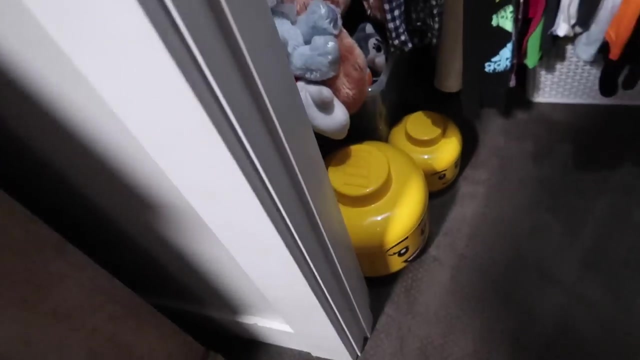 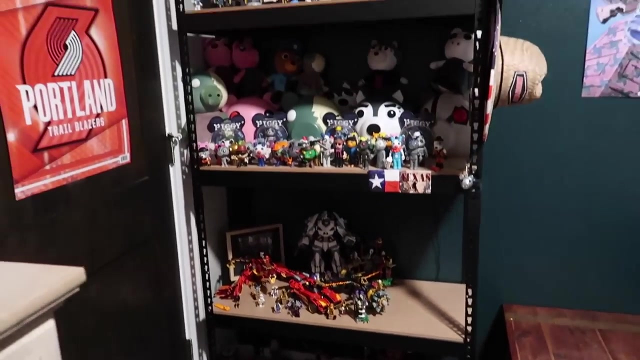 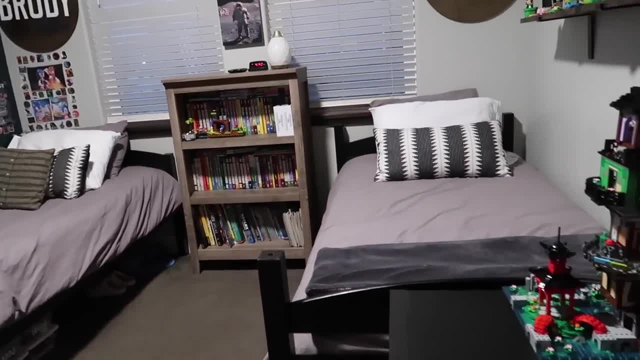 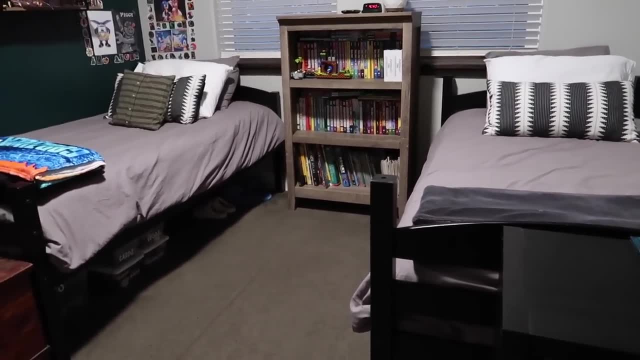 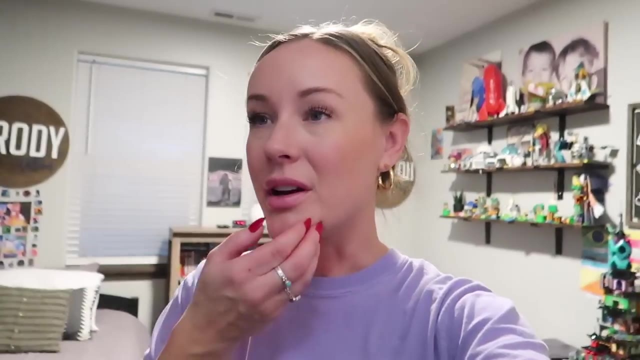 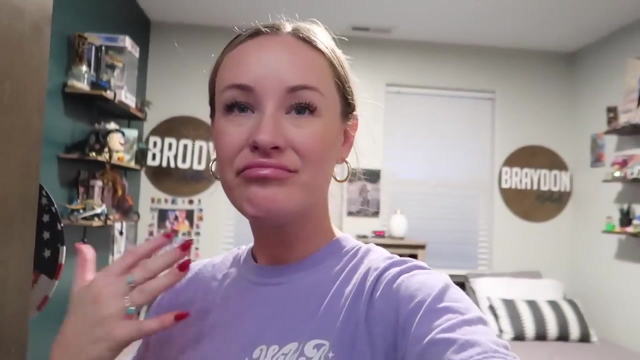 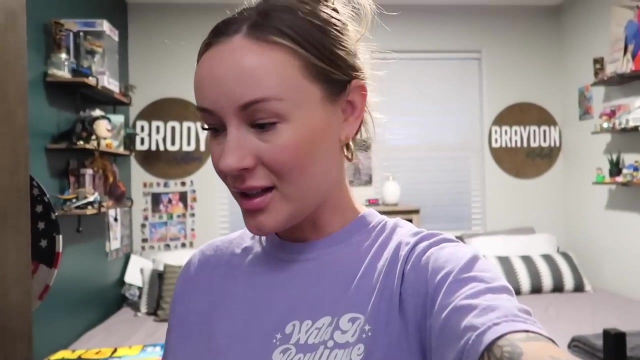